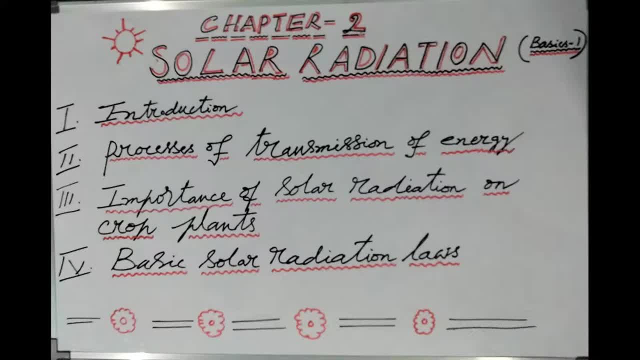 Dear and beloved students, welcome to our class on solar radiation. This is the second chapter of our course: agro-metrology and climate change. Now, before I actually start the class, until all our students enter and then take their seats, I just would like to tell a small story. It is a very simple. 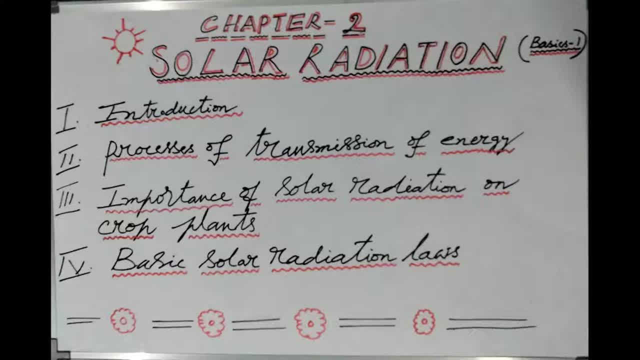 one, Some boys were playing near a pond. They saw a number of frogs in the water- number of frogs in the water- and began to pet them with stones. They killed several of them. After a while, one of the frogs, lifting his head out of the water, cried out at the boys. 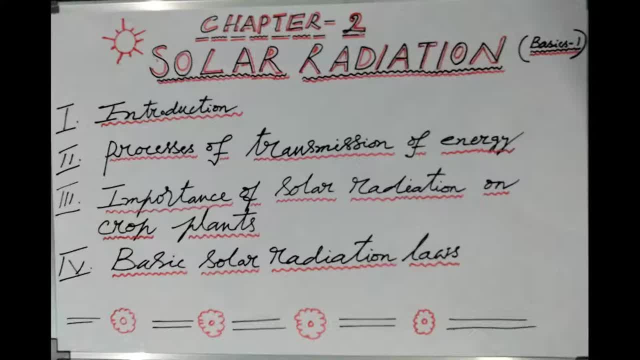 I pray, I pray, I pray. stop, stop, stop My boys. I pray, stop petting stones on us. What is sport to you is death to us. The moral is: one man's pleasure may be another man's pain. 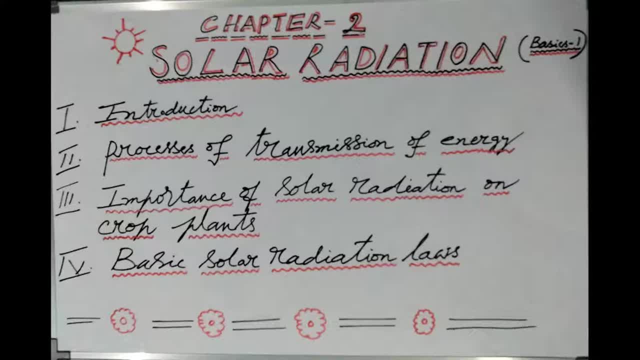 Okay now. So let us go into the class. Today, as I said in the beginning of this class, we are going to discuss the second chapter of our course, that is, solar radiation. Solar radiation is the primary source of energy on the earth and life depends on it. 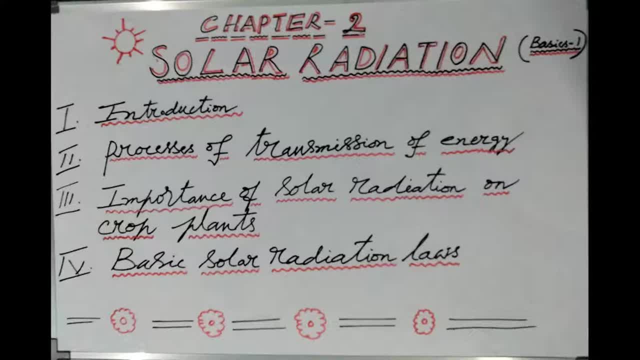 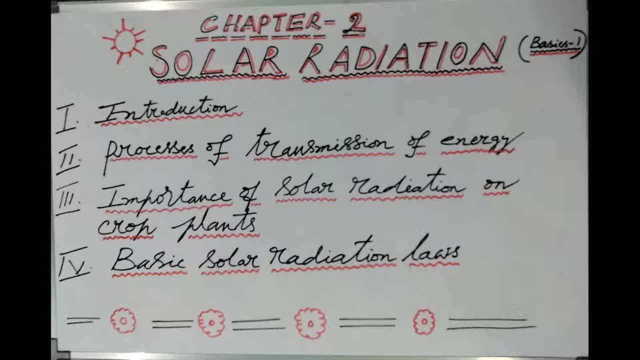 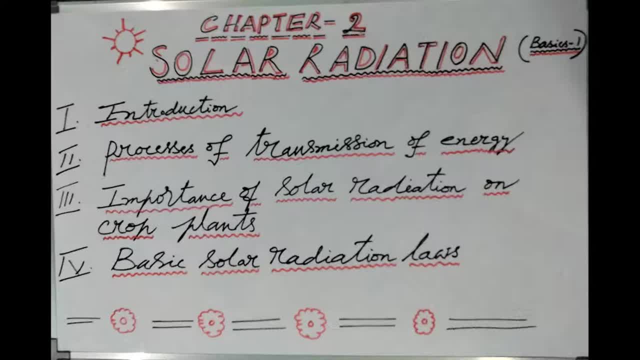 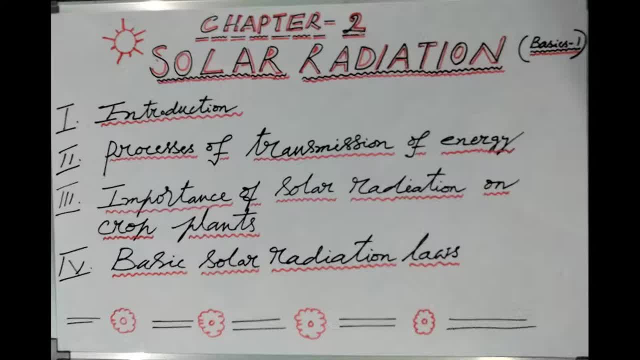 The processes of transmission of energy. One: radiation. This is the process of transmission of energy from one body to another without the aid of a material medium. There is no material medium in it, Neither solid nor liquid, Anything, Anything, Anything. Therefore, radiation is the process of transmission of energy from one body to another without the aid of a material medium. Example is the energy transmission through space, from the sun to the earth. 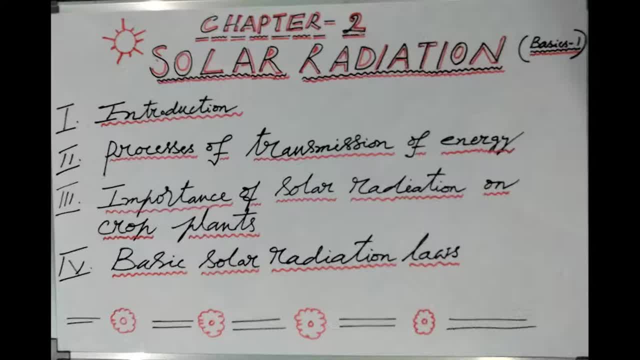 Okay, The second process of transmission of energy. The third process of transmission of energy is conduction. The process of heat transfer through matter without the actual movement of the molecules, of the substances or matter is known as conduction. Once again, I would like to repeat. 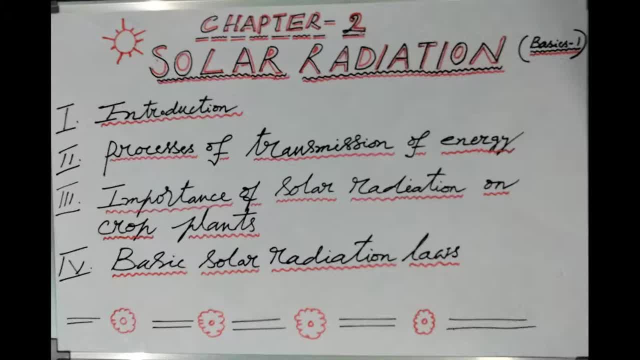 The process of heat transfer through matter without the actual movement of the substances or matter is known as conduction. Once again, I would like to repeat. The process of heat transfer through matter without the actual movement of the molecules of the substances or matter is known as conduction. 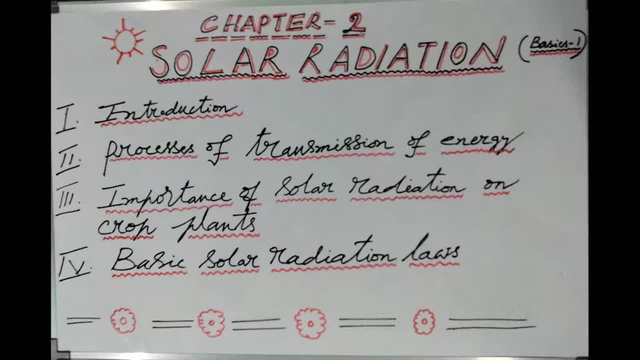 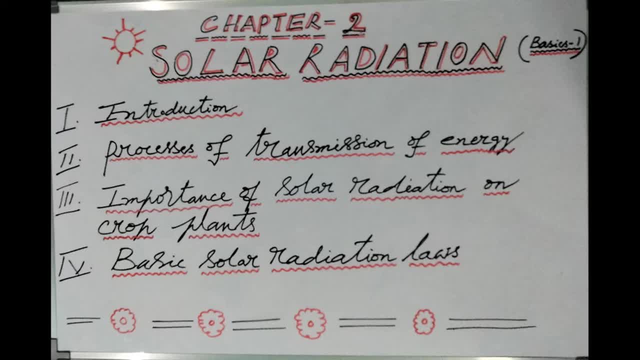 Heat flows from the warmer to cooler part of any body so that the temperatures between them are equalized. Heat flows from the warmer to cooler part of any body so that the temperatures between them are equalized. black body is inversely proportional to its absolute temperature. for your benefit, so very. 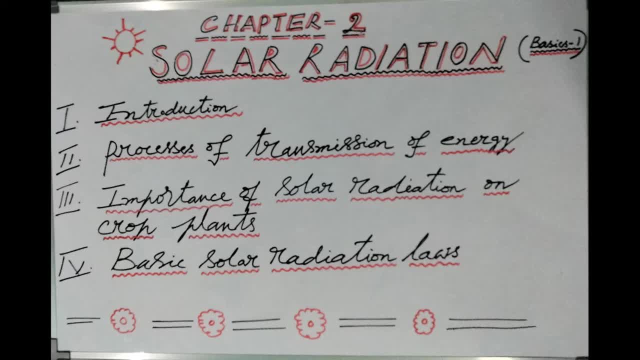 interesting, very simple. the wavelength of the maximum intensity of emission from a radiating black body is inversely proportional to its absolute temperature. for small example or explanation: if the temperature of a body is high, radiation maximum is displaced towards the shorter wavelengths. for the surface temperature of, say, for example, 5793 degrees kelvin, evaluated for the sun. 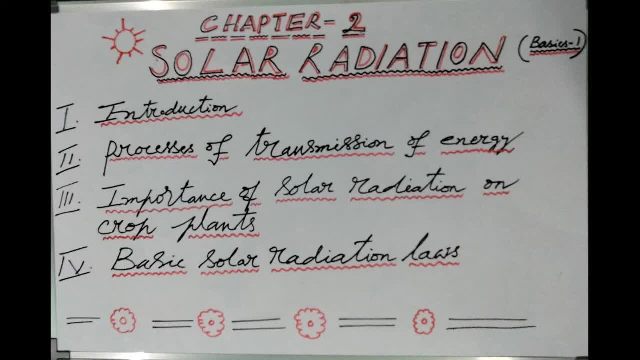 lambda maximum is 0.5. the most intense solar radiation occurs in the blue green rain of the界 M e value. as if its free play, it decays with the same frequency. it is fact. visible light, the wavelength of maximum intensity of radiation for the Earth's.